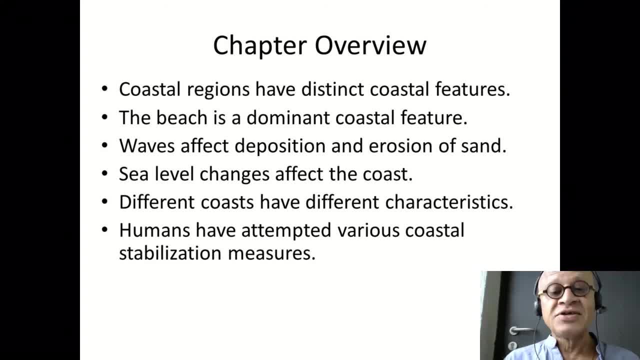 Sea level rise is constantly a buzzword that we are using, which is now pretty serious because it's not only rising, but the rate of rise is accelerating. So sea level rise is accelerating in many places. So that's always Something that is of great concern at the coast, especially if you have built something very close to the coast, or if it's a port, it's a naval station, and so on and so forth. 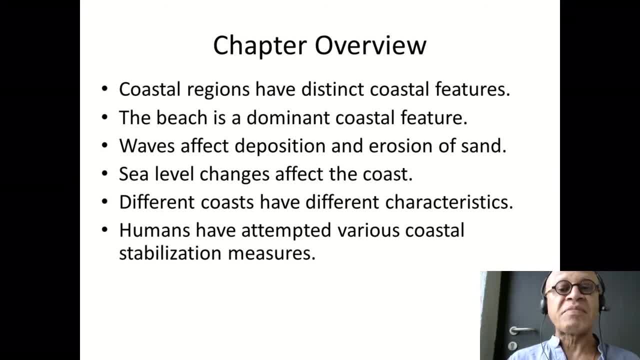 We will see how different the coasts are and what makes them different, and how human beings create the processes that favor erosion or their natural processes, and how human beings want to prevent them to be able to live close to the coasts. These are kind of the things that we will look at in this chapter. 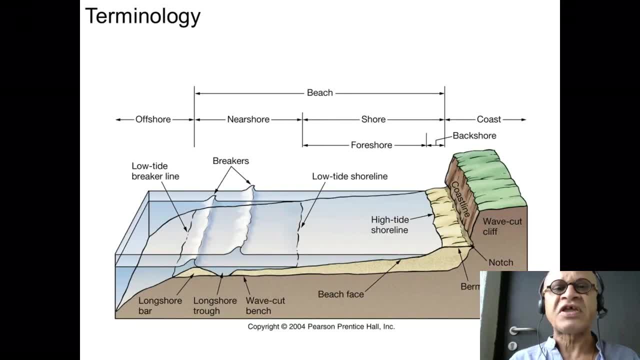 Defining the coastal regions better. to just look at this figure here, This is kind of idealized. Obviously, not every coast will have all these features, but you will recognize most of them. So there is a broad definition of the beach. So when we go to the beach we typically say: 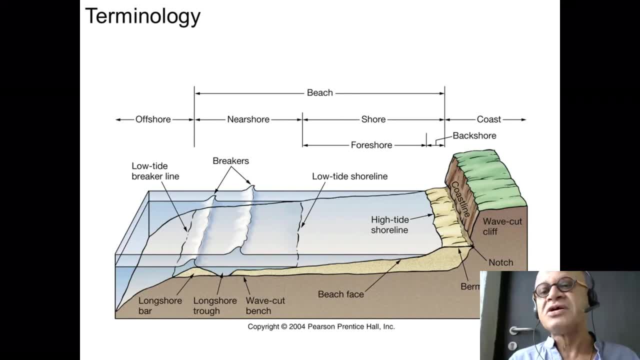 the sandy part is the beach. Actually, technically speaking, that is what is called a berm. okay, Berm is the sandy part in this pure scientific definition, And then the entire extent of the coastline down to what is called a longshore bar, which is related to the tidal action, is called the beach. 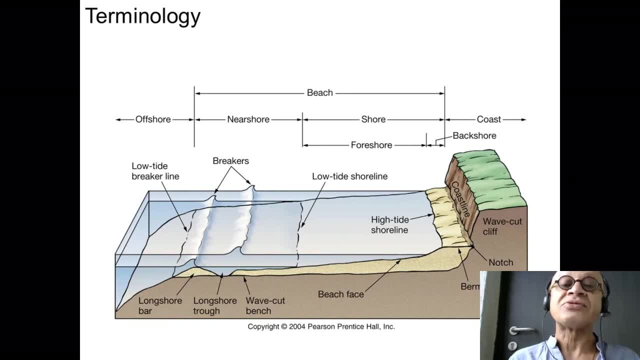 And beyond this low tide breakage. This line, as I said, is not always defined at all the coasts. It depends on many other factors. It is called the offshore And towards the coast from this longshore bar, the low tide breaker line. 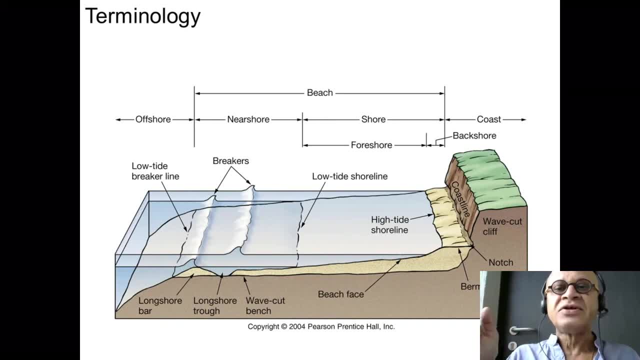 you have the nearshore and the foreshore, okay, So the shore includes the foreshore and the backshore, The backshore includes the berm and so on. Basically, there is a seasonality here. Typically you have a high tide line and a low tide line, And we will see the processes which bring the sand in. 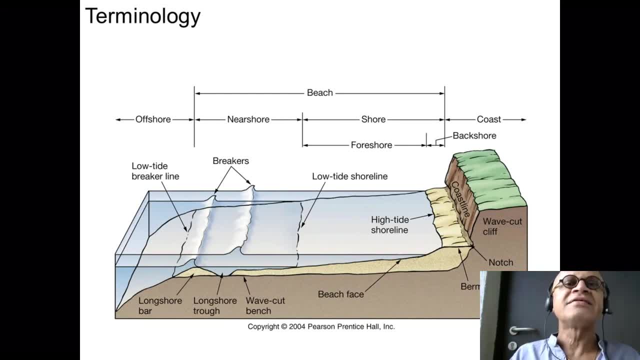 and take the sand out, And there is a seasonal dependence of the wave energy, So the beach itself can look very different when you go away from the tropics. In the tropics you don't have a very strong seasonality right. Pretty much the whole year is nice and warm. This is why people like to come to the beach in the tropics- beaches in the tropics in the winter, correct? So avoid the winter where they are in the mid-latitudes and find some nice tropical beaches okay. 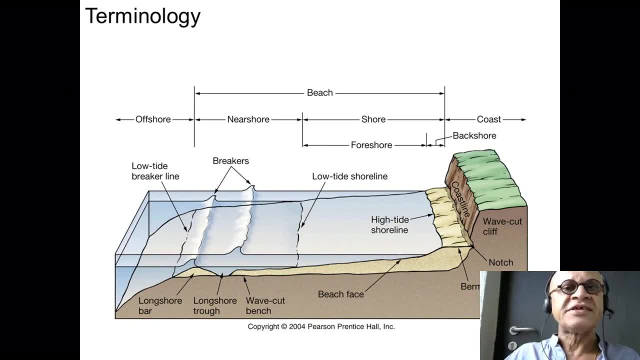 Coastline is basically the extent to which the marine processes, the coastal processes, affect things. So you can think of it as how far the sea salt would go in, how far the sea breeze would go in, and so on. There are many coastal features that you can find. It can go for miles, correct? 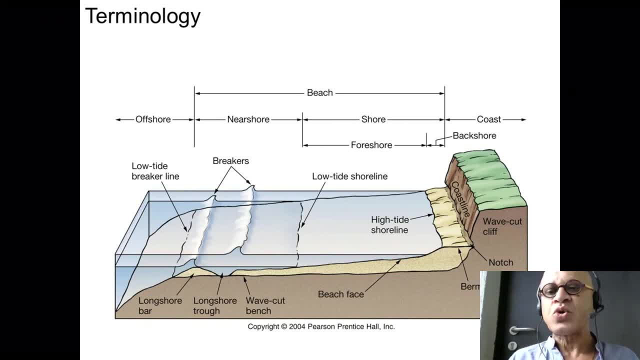 Okay, so you have the high tide shoreline to which the water sloshes up during the high tides, And within the water column you have the beach face. So you have the wave cut bench longshore trough. So, essentially, the sand is being moved onto the beach during the high tide. 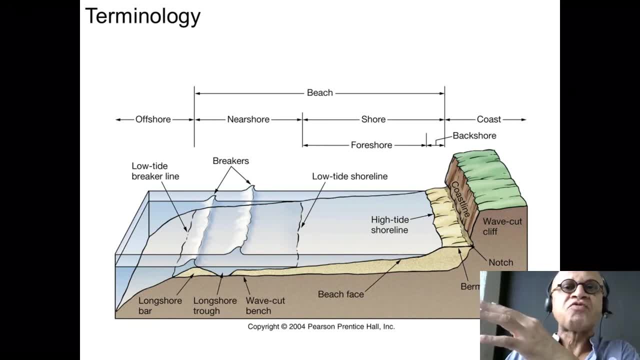 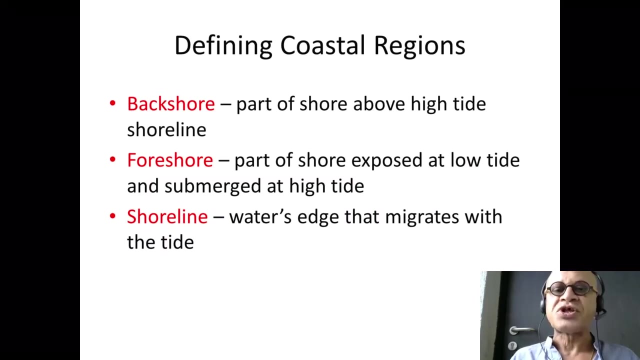 And then it goes onto the beach. during the mild summer season, when the wave energy is low, Waves are milder And then wash out the sand during the other seasons. Again, you don't have to remember all the terminologies, but the terms like backshore, foreshore and shoreline are used in common languages. 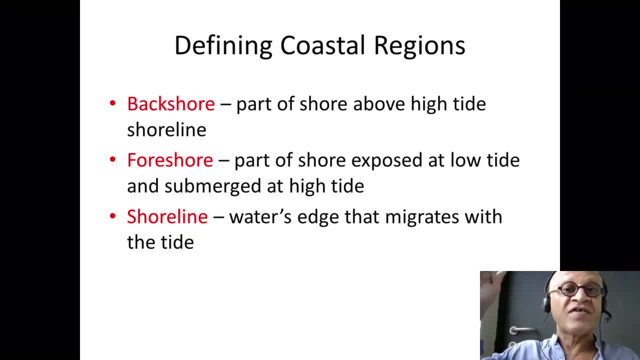 Okay, so backshore is part of the shore, above the high line, the tide line, And foreshore is the part of the shore. that's extreme. It's exposed at low tides, So it's submerged during the high tide. Okay, so shoreline is essentially the water's edge that migrates with the tide. 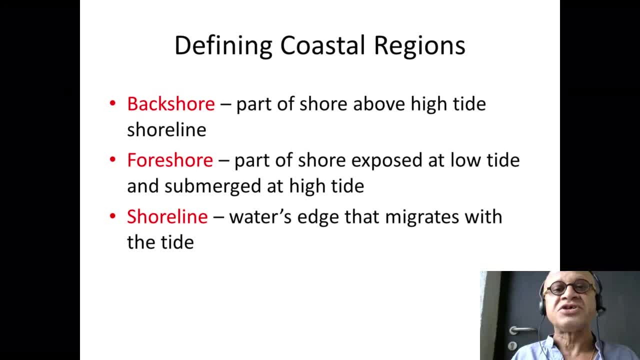 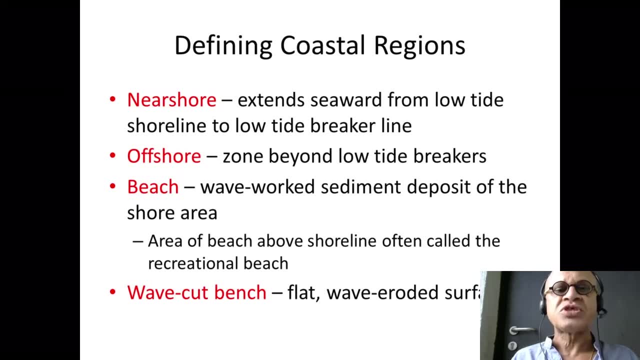 High tide line, low tide line, that is the shoreline with the backshore and the foreshore. Okay, so you also have the nearshore, the offshore, the beach and the wave cut bench Again. you cannot find them exactly.